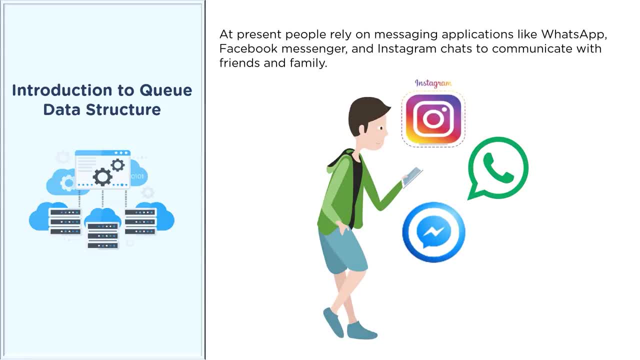 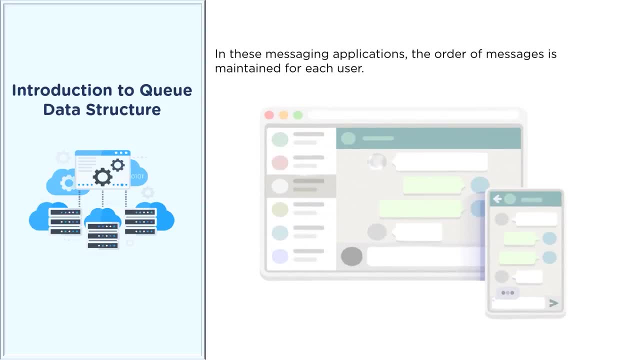 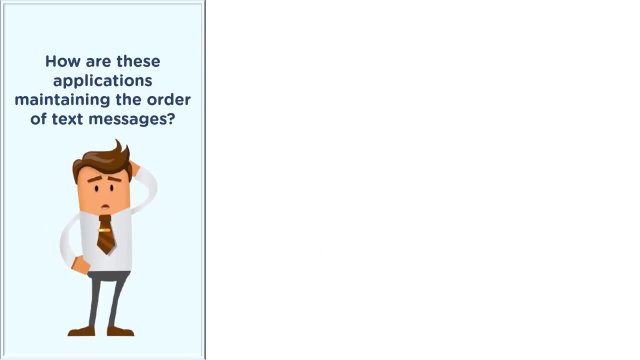 messaging applications like WhatsApp, Facebook Messenger, Instagram, And while using them, you must have observed that the person you are trying to communicate with receives messages in the same order as you have sent them. Now the question that arises here is: how is this happening? How are these applications maintaining the order? 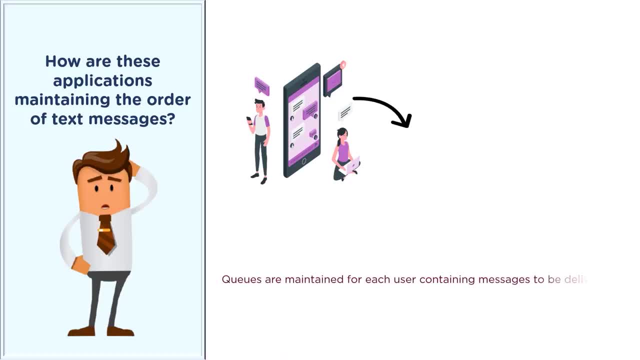 of these text messages, And the solution to these questions Bring us to queue. Basically, in these applications, a queue is maintained for each user containing the messages to be delivered to the user When the user connects to the network, all the text messages in the queue gets delivered. 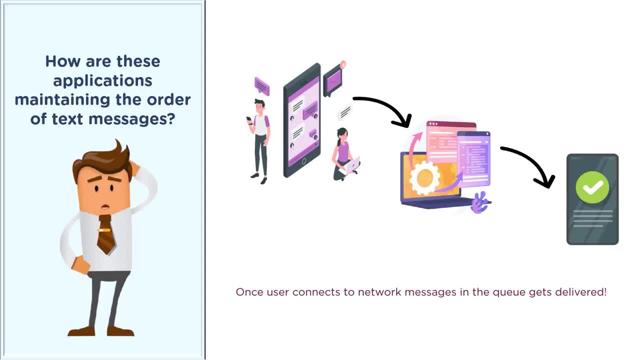 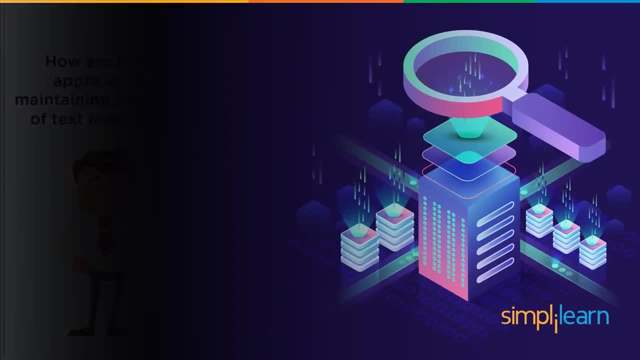 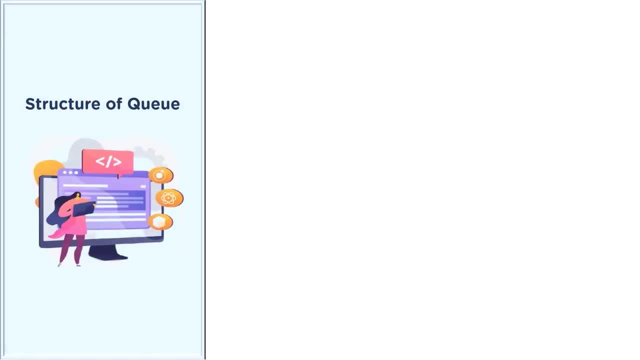 And once the messages are delivered, empty queues get deleted. This example clearly illustrates the importance of data structures. So let's dive further and understand the structure of the queue in depth, But before doing that, let's look at a real-life example of queues to understand it more clearly. 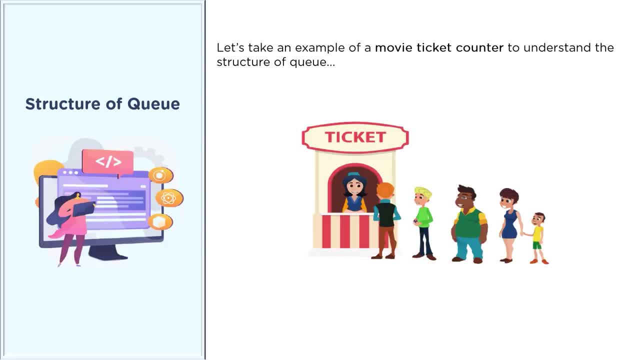 The most common and relevant example of a queue is a movie ticket counter. In the movie ticket counter, you must have observe that both of its ends remain open. Also, these ends are fixed with the help of barricades, And that is why no one can enter in between these ticket lines. 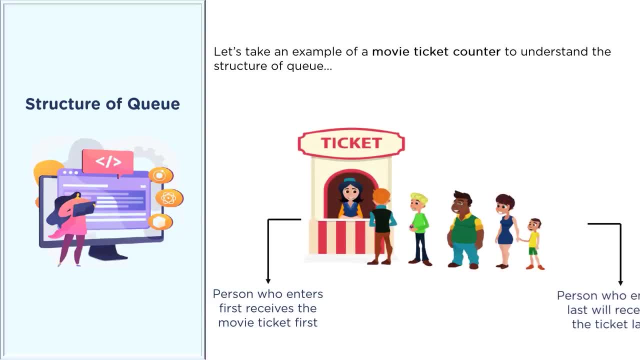 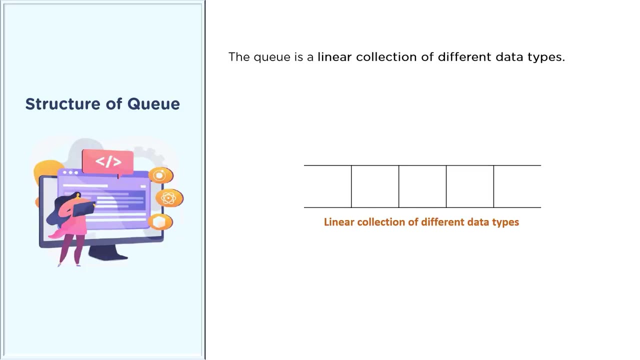 Additionally, the person who enters first receives a ticket first, and the person who enters last will obviously get served at last. Queues and data structure resembles all these properties of a movie ticket counter, which makes them better at creating virtual first-come, first-served systems. Basically, they are defined as a linear collection of different data types. 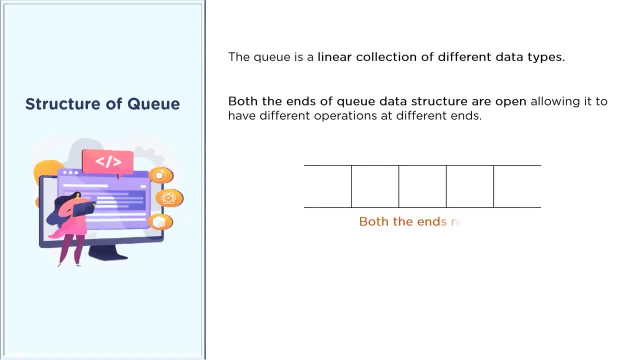 that allow insertion at one end and deletion at another. Unlike any other data structure, the queue ends remain open, allowing it to have different functionalities at both ends: The end at which insertion takes place is called rear and the end at which deletion takes place. 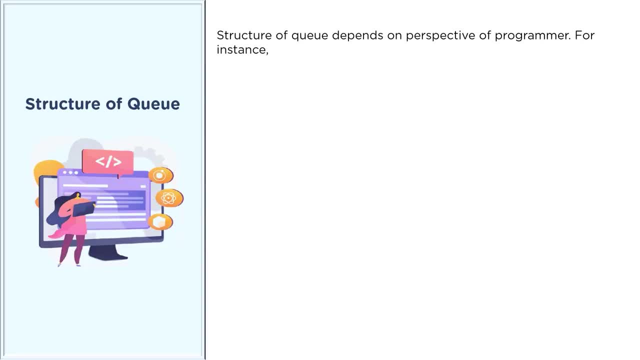 is known as front. Furthermore, there are two approaches to consider the structure of the queue, and both of them depend on the approach of the programmer. That means being a programmer. if you consider the left end as front, then your rear end is the front and the left end is the back. 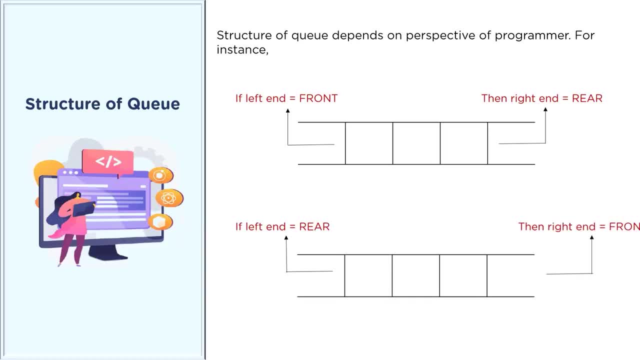 The rear node will be at right end. Otherwise, if you consider the left end as rear, then the right end will be your queue's front node. Unlike arrays and linked lists, elements in the queue cannot be operated from their respective locations. Here they can only be operated from the front or rear. 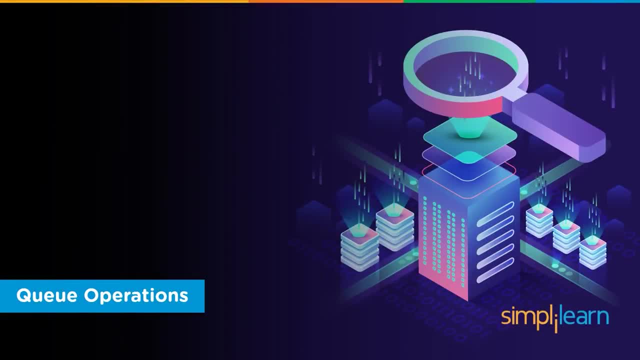 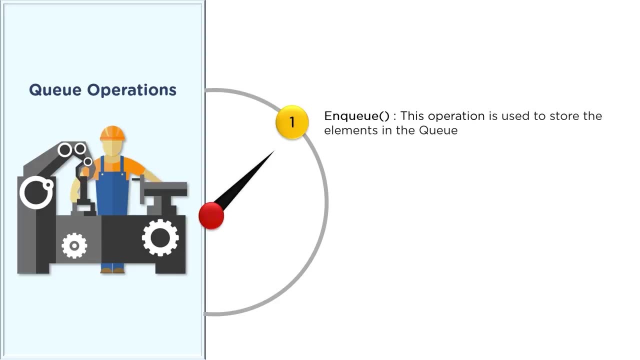 position. Moving on, let's discuss the operations in queue data structures one by one. The first operation is enqueue. It is used to store the elements in the queue. Next up is dequeue. This operation is used for removing them. Further, we have isfull and isnull operations. 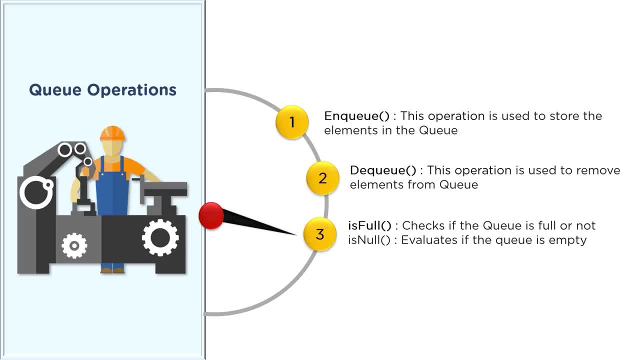 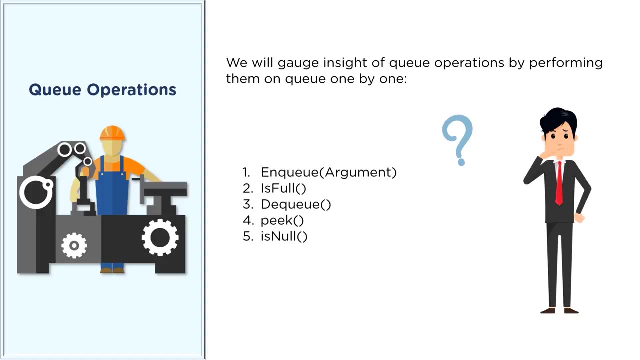 Isfull function scrutinizes if the queue is full or not, and the isnull operation evaluates if the queue is empty. We also have a peek operation that helps you get the element from the front of the queue without removing it. Let's now understand how these operations work with the help of the following examples. 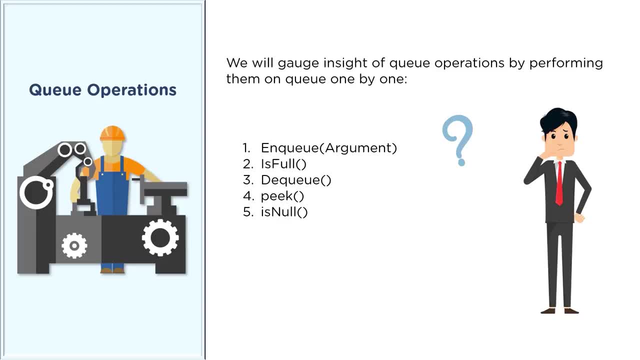 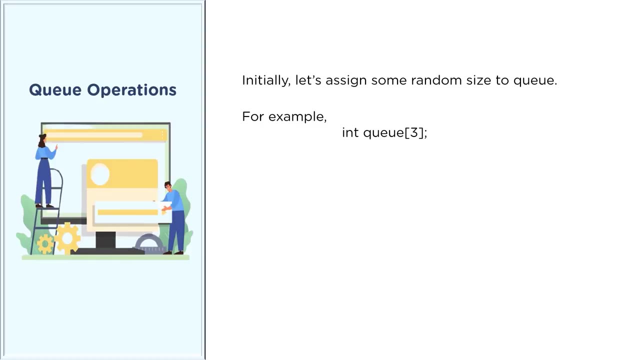 Here we will look at enqueue5,, enqueue1,, enqueue-2,, then isfull, then dequeue, peek and isnull. But before explaining these operations it's essential that we initialize the queue data structure by assigning some random size to it, For example, int. queue of 3.. By this declaration, 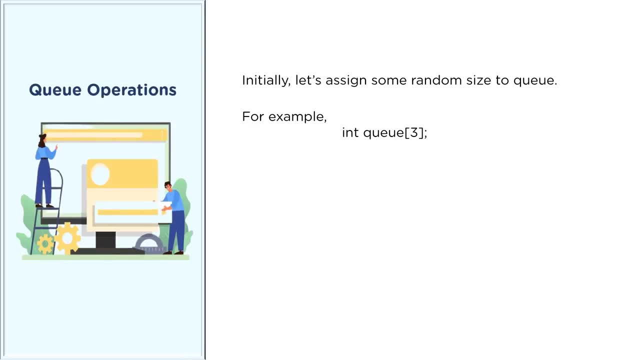 we are assigning only 3 spaces for insertion in queue. Also, at this phase there is no element in the queue. There is no particular type of inside node that usually associates q and an outras. You cannot add the total input space in the queue as it's empty. So both the front node and rare node will point. 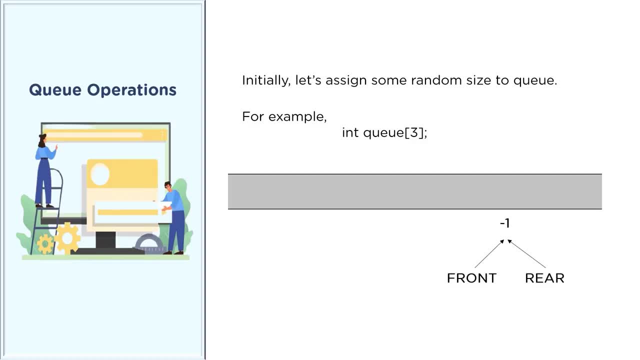 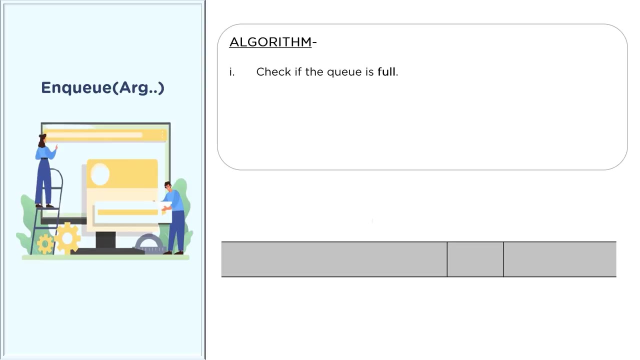 to the same location with null memory space in the storage system. Let's consider that null index to be minus 1 for ease of our convention. Now the first operation on our list is enqueue5.. As we discussed previously, enqueue operation is nothing but the insertion of data into a queue. 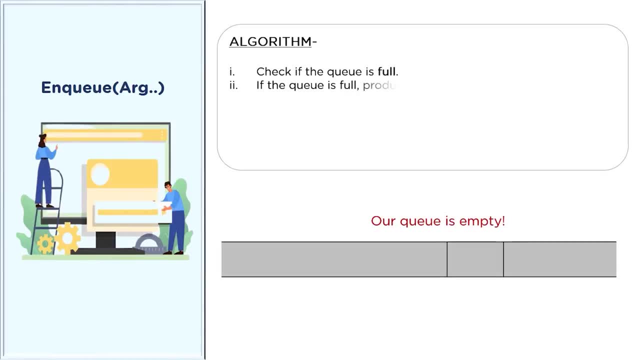 data structure. It begins with checking if the queue is full or not. If the queue is full, then the previously assigned memory is saving. the late queue is completely filled with data elements, So insertion would not be possible. This is also known as overflow error in terms of programming. But as our queue is empty, so the insertion 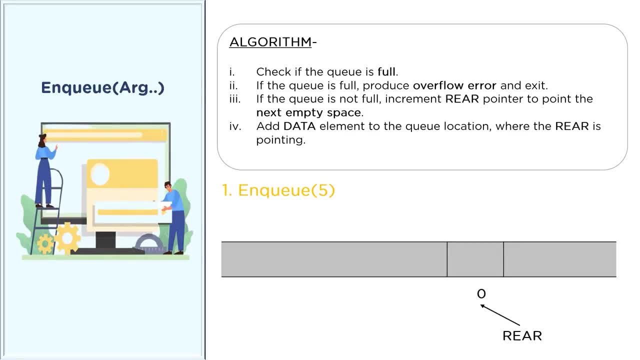 can be performed here. For that we have to increment the rare pointer to index 0 from index minus 1.. And once we do that, the data element phi will be added to the queue. Also, for front insertion, both front and rare will point to the same location, as there is only. 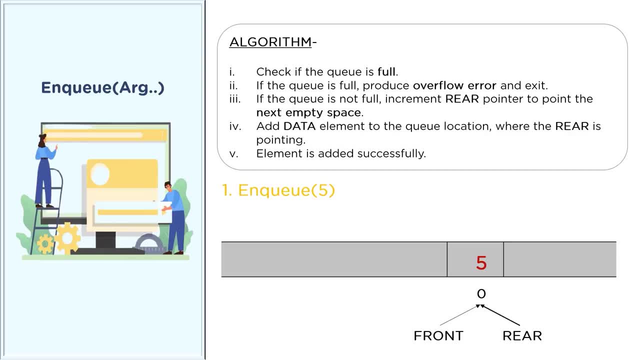 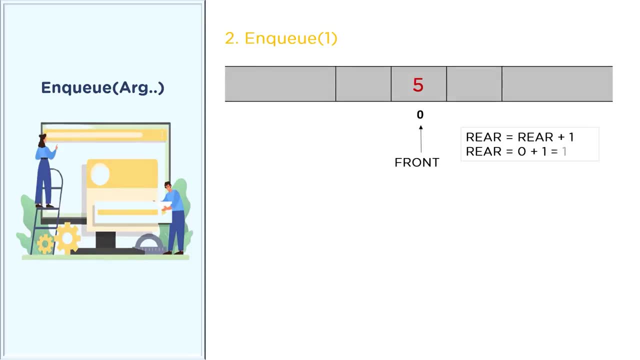 one element present in this queue. Let's insert two more elements into this queue with the operations nq 1 and nq minus 2.. For that we have to increment the rare pointer to the next index, which will be 1.. Now, as the pointer is incremented, so the data will be entered. 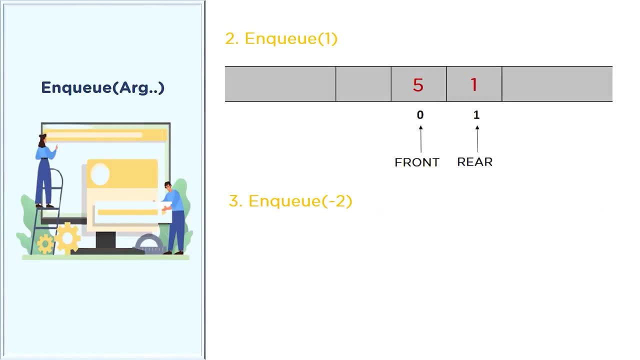 into this position. Next up is nq minus 2.. Again, we have to follow the same process of incrementing the rare pointer. We will increment the rare pointer to point towards the next index index, that is, index 2, and hence the data element with value minus 2 will be entered here. the next: 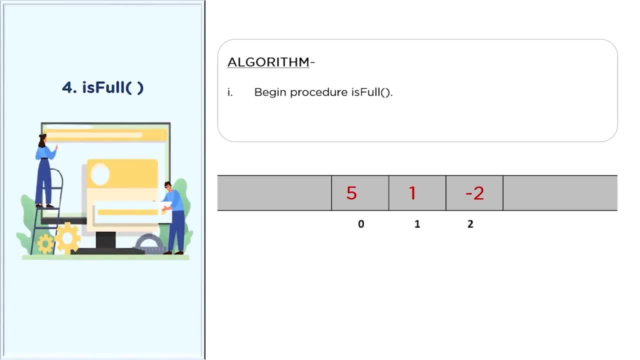 operation on our list is is full. in this operation, if the rare pointer points to the max size, then the queue is considered to be full, as there is no space left for insertion. in our case, the max size of our queue is 12 bytes. additionally, we are considering to enter only three integer. 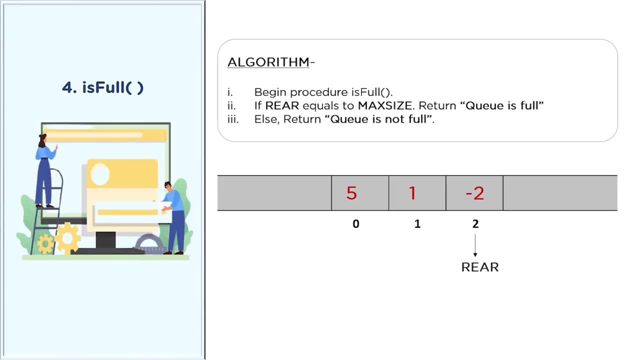 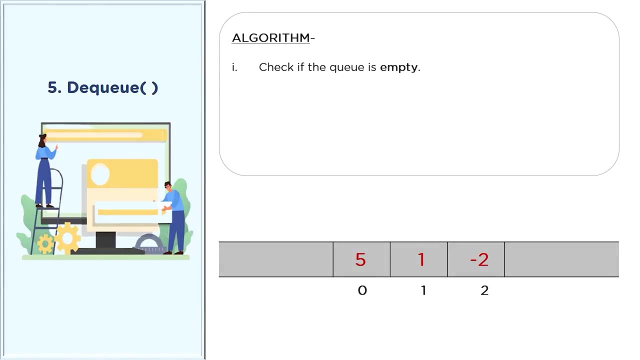 elements and one integer data element takes 4 bytes of the memory space. that means three integer elements will take 12 bytes. hence this function will prompt. q is full on the screen. now we will discuss the dq operation. if we want to access data from a queue, we have to perform: 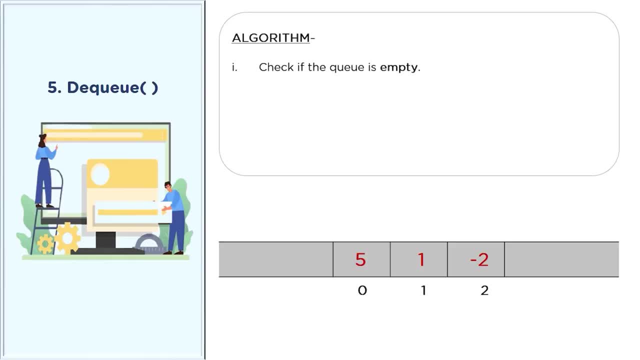 two subtasks. the first one is access the data where the front is pointing and another is to remove the data after access and this complete process is called as dq operation. the first data element takes 4 bytes of the memory space. that means 3 integer elements will take 12 bytes. 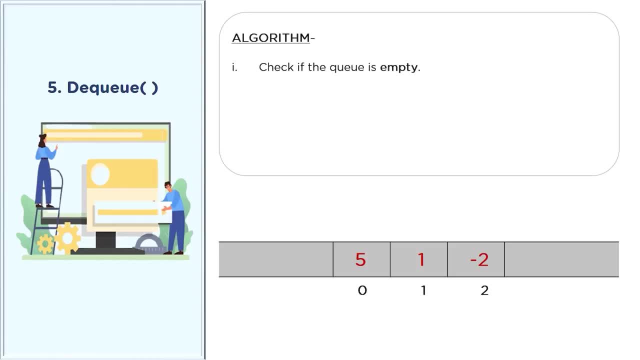 step of this operation is to check if the queue is empty. if the queue is empty, then there is no element available for deletion. this is a case of underflow error, but as our queue is not empty, we can proceed with the next steps. we will be accessing data from: 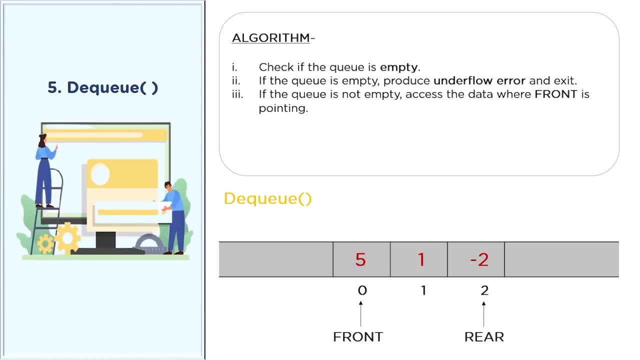 the front node and later we will be incrementing the front pointer in order to remove the link to the previous node, so that the data gets removed. now, front will point to the index 1. thus the data value phi will be removed from the queue and will also be prompted on the screen. 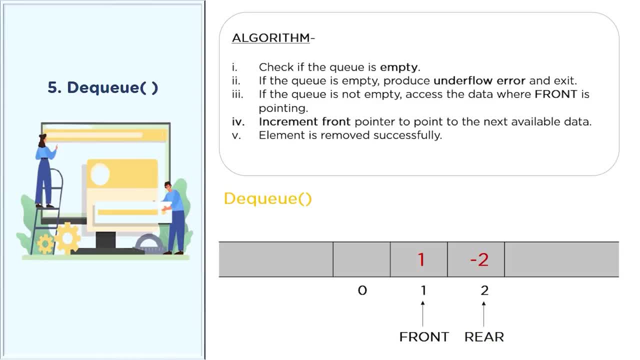 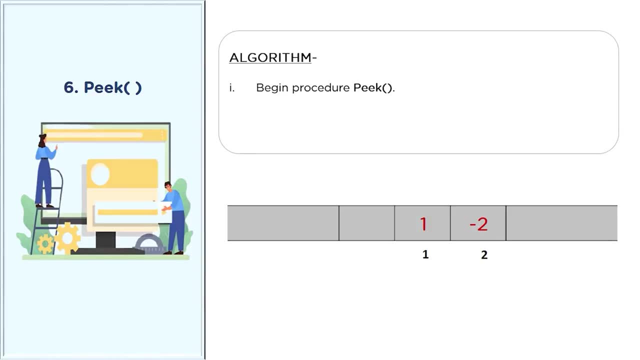 therefore, this function comes with an integer return type. next up is peak operation. in this operation, element at the front node will be accessed without deleting it. the algorithm for this operation begins with checking if the queue is empty or not. if the queue is not empty, then data at the front node will be accessed with 10% of the data element. 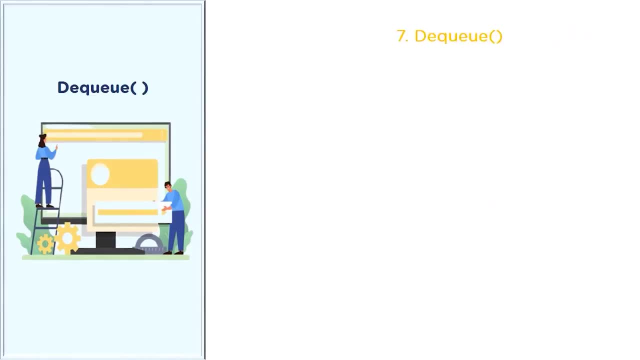 temporary variable and printed on the screen. advancing further, let's perform two more dq operations here. first is dq of 1 and another one is dq of minus 2.. the data at the front node will be accessed primarily and the front pointer will be incremented to point to the next data element. 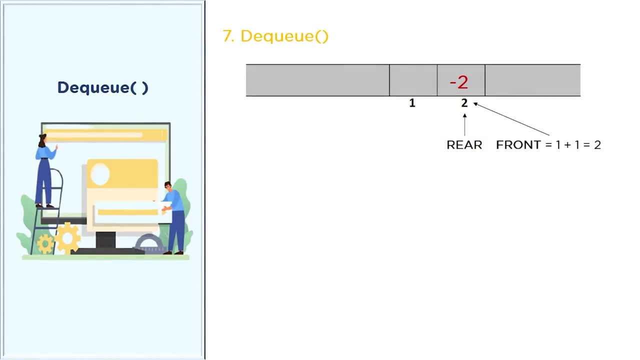 when we do the pointer incrementation, the link to the previous node gets removed, which results in data deletion. similarly, we will perform a dq of minus 2 operation here. now the front will be pointed to null memory space, as there is no element left in our queue. 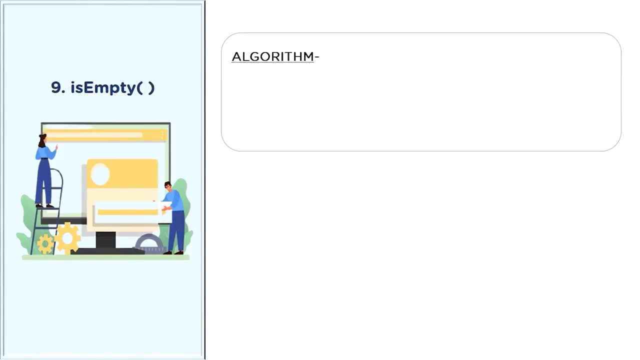 and the data minus 2 will be removed. the last operation on our list is is empty. this function checks if the queue is empty or not. in the previous procedure we mentioned that if the front points to the null memory space, then the queue is empty and in our case, 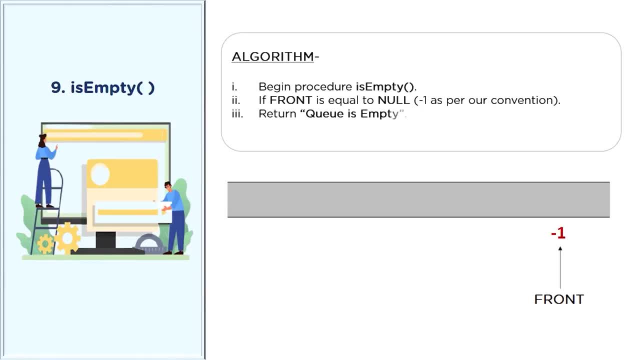 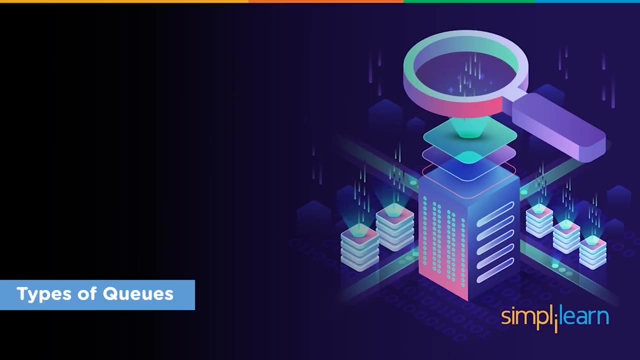 the front is already pointing to minus one, so the output of this function will be: q is empty. this is all about operations in the queue. i hope that you all are clear with these operations. next we will discuss different types of queues and their structures at a glance. 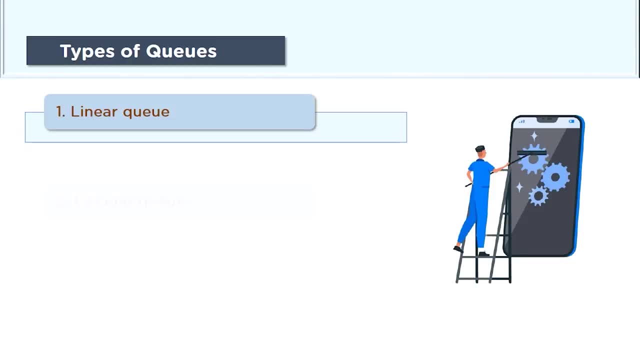 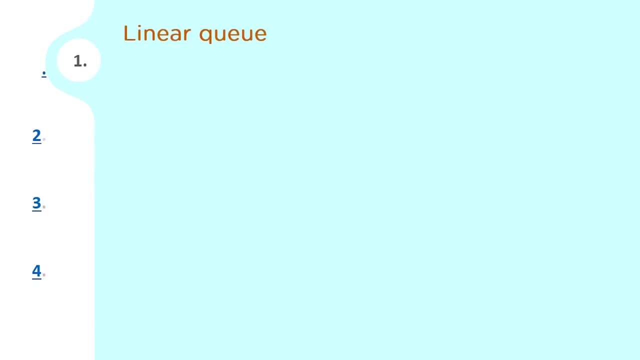 basically, there are four types of queues: linear queue, circular queue, priority queue and double ended queue. the structure which we have discussed till this time is that of a linear queue, so now we will move on to circular q. the circular q is almost similar to the linear q. 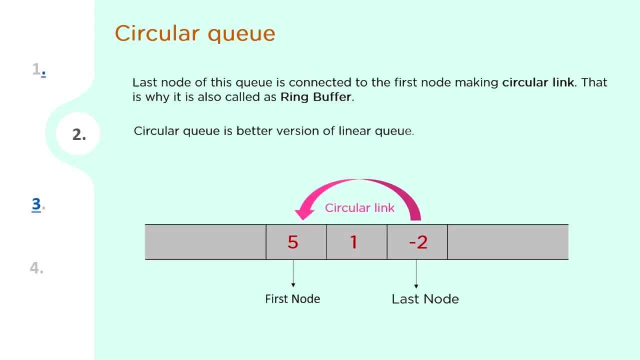 the last node of this queue is connected to the first. It is also known as ring buffer, as all the ends are connected to another end. Additionally, this circular queue is a better version of the linear queue as it removes the drawback of insertion in the linear queue. 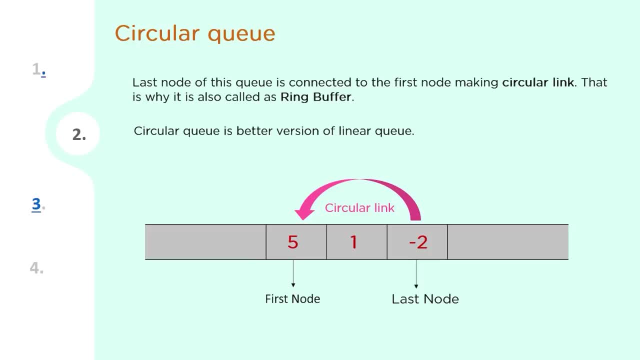 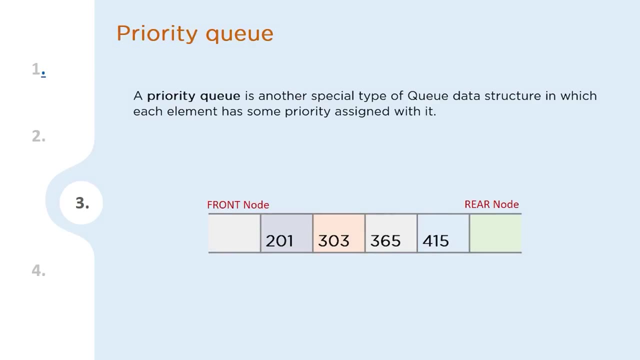 The empty space available in a circular queue can be filled with the new element by simply incrementing the value of the rare position. We will learn about this in detail in our further sessions. A priority queue is another special type of queue data structure in which each element has some priority assigned with it Based. 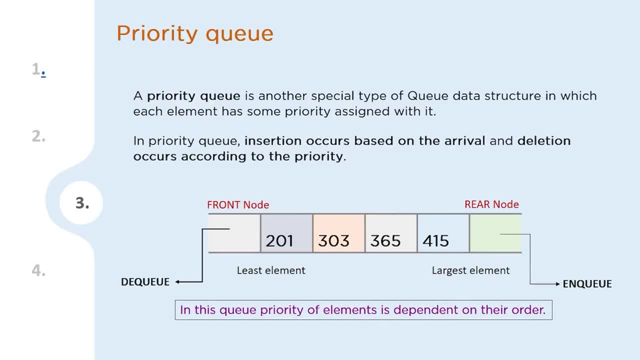 on the priority of each element. the elements are arranged in a priority queue. If the elements occur with the same priority, then they are served according to the first-in-first-out principle. In the priority queue, the insertion occurs based on the arrival, while the deletion 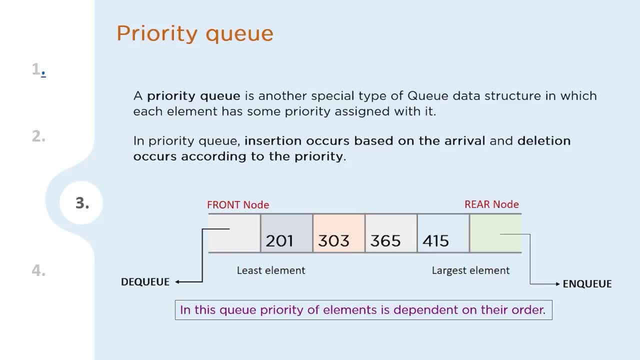 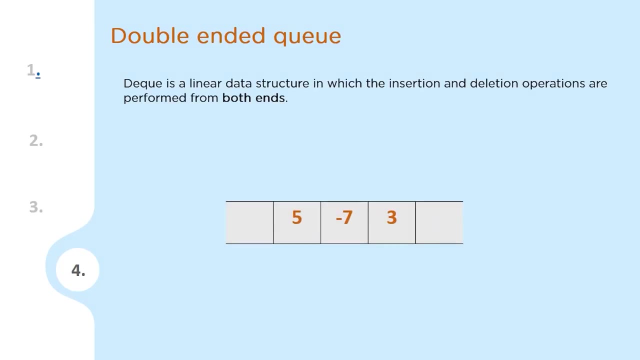 occurs based on the priority. The above figure shows that the highest priority element comes first and the elements of the same priority are arranged based on the first-in-first-out structure. The last type of queue is DQ. DQ is a linear data structure in which the insertion and 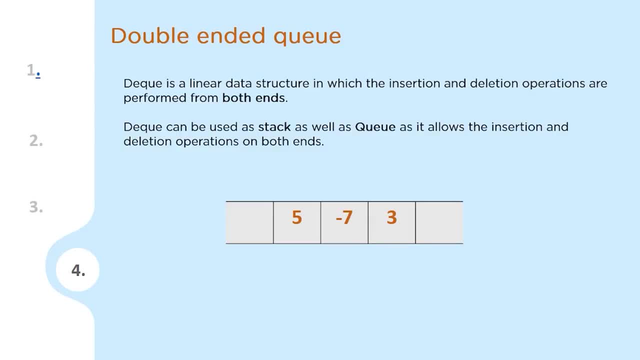 deletion operations are performed from both the ends. We can say that DQ is a generalized version of the queue. DQ can be used as stack as well as queue, as it allows the insertion and deletion operations on both the ends. If the insertion takes place at one end and deletion at another, then that DQ is known. 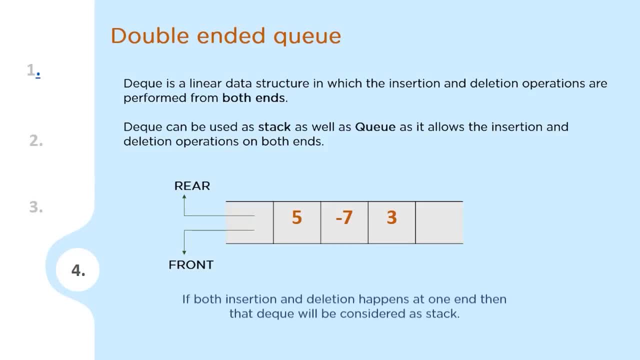 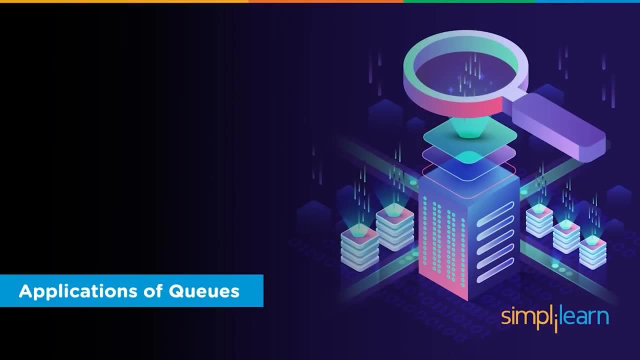 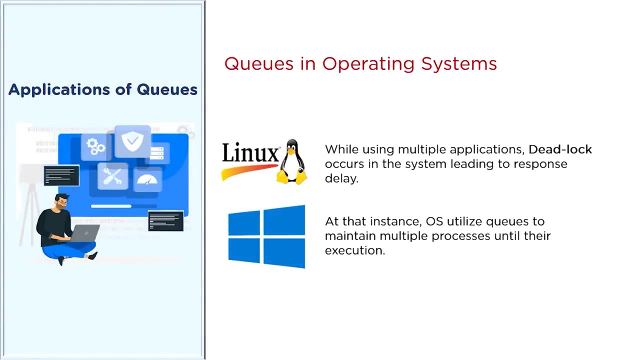 as a linear queue And if both addition and deletion are performed at a single end, then that DQ is called stack. Advancing further, let's discuss some applications of queues to gauge and insight into the importance of queues. The queue data structure is used in computers, printers and applications to utilize the benefits. 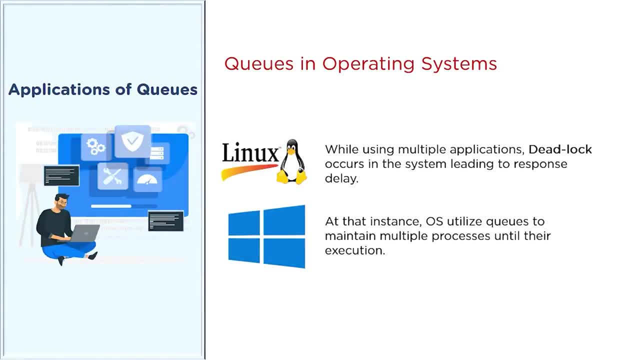 of the first-come-first-served technique, Because whenever you work on documents or PPTs, you must have observed that whichever key you press on the keyboard appears in the exact same order on the screen. But when your processor is too busy with other tasks, you might notice that the keys you press appear. 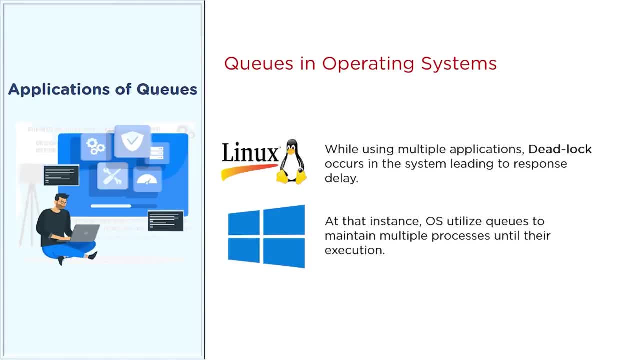 on the screen with some delay after you press them. Basically those keys are stored in queue and when the processor becomes free it processes in the order the keys are pressed. That means the key pressed first will be written in a Word document first. So this is how computers use a queue to 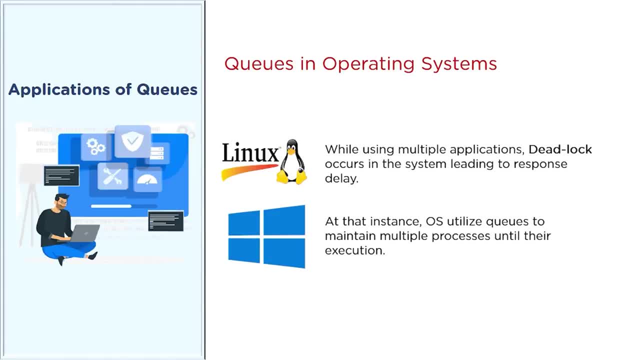 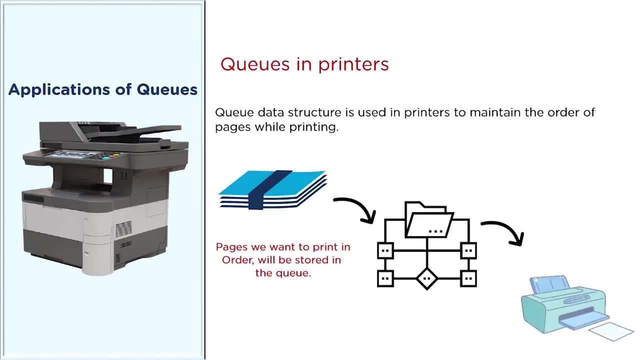 eliminate deadlocks when multiple processors are in a ready state. Next up is printers. A queue data structure is used in printers to maintain the order of pages while printing. That means the pages are stored in a queue in the order that you want to print them. 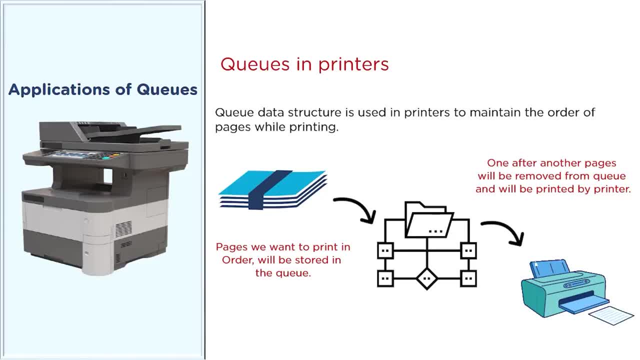 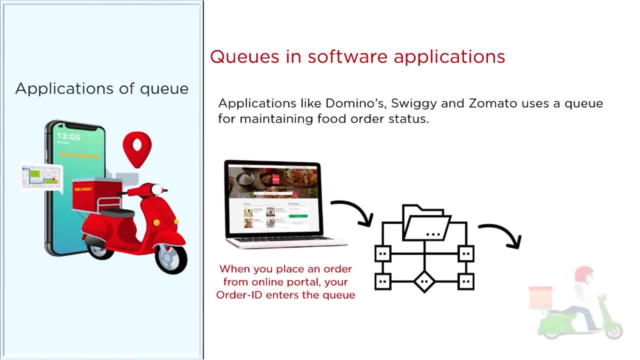 and once the page is removed from an ordered queue, it gets printed. Another most common application of queue data structure is their usage in web or mobile apps. Applications like Dominos, Swiggy, Ussr and a bunch more are used for a regular kind of